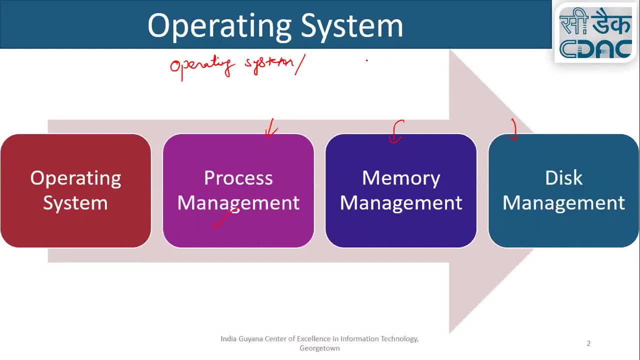 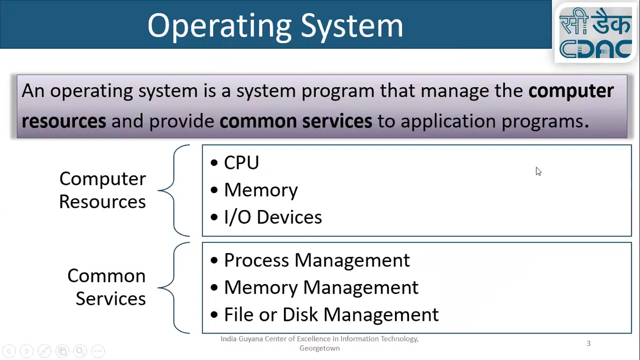 area for today is the process management. Yesterday we already completed this device driver and utility shockwares. Okay, Yes, sir. So let me move to the next slide. So this is the slide from my previous slides. It defines what is updating system. So an updating 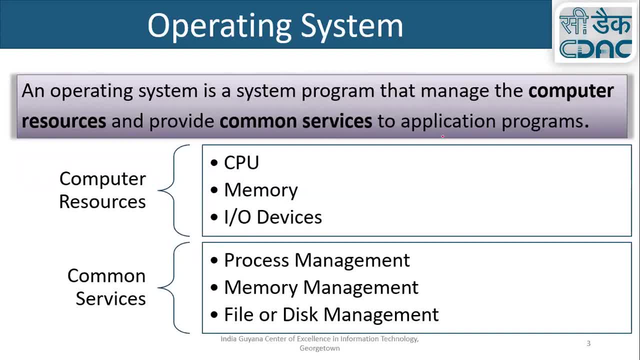 system is a system that is used to update the system. So it's a system that is used to update the system. So it's a system that is used to update the system. So it's a system program that manages the computer resources. So this is the two thing most important thing. 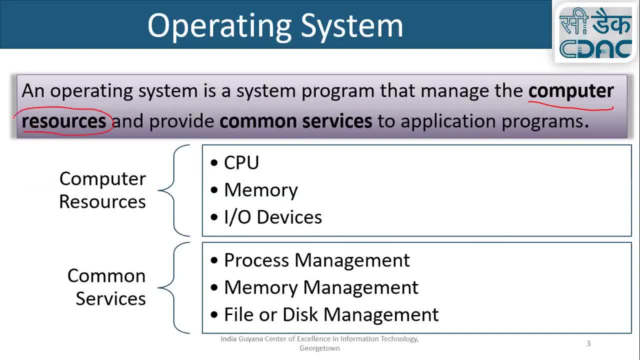 here. One is that manage the computer resources, Okay, And provide common services, Okay. So what are the different resources inside your computer system? If anybody asks what are the different resources, So some most important resources: CPU, your processor, the CPU, your. 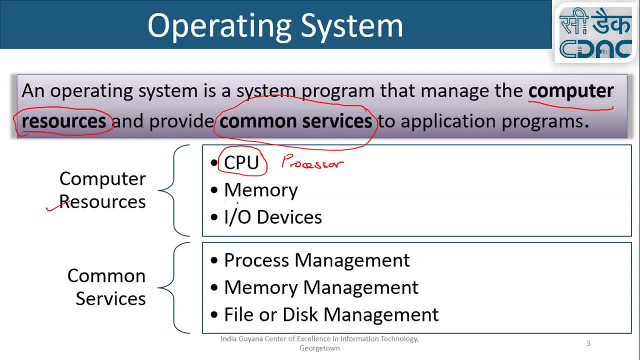 processor, the CPU, your processor, the CPU, your processor, and then your memory. Here the memory means your RAM, Okay, And your cache memory, of course, And then IO devices. It's like your hard disk, your display or monitor Okay, Your keyboard Okay, And network. 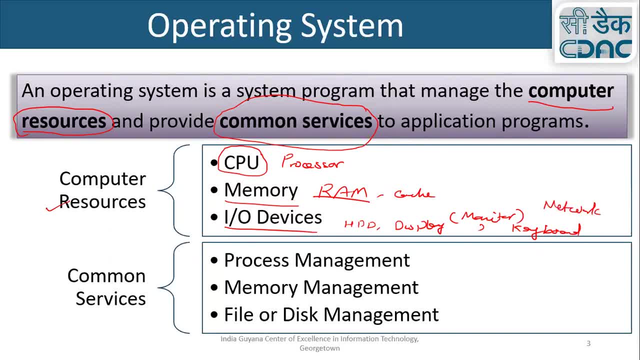 And your laptop, Okay, Your computer, Okay, So so, these are all the different resources, Okay, And appleting system. manage these resources, How and while managing these resources, it provide you with some common services, Okay, So when, please remember this, please remember. 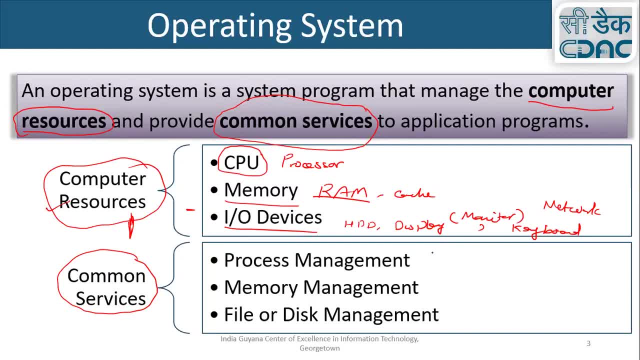 this sequence here: Uh, when your Uh, Uh- operating system Manages the CPU. Okay, this is acting as a process. This is known as process management. Okay, basically, it's dealing with their CPU. Okay, so when you're operating operating system. 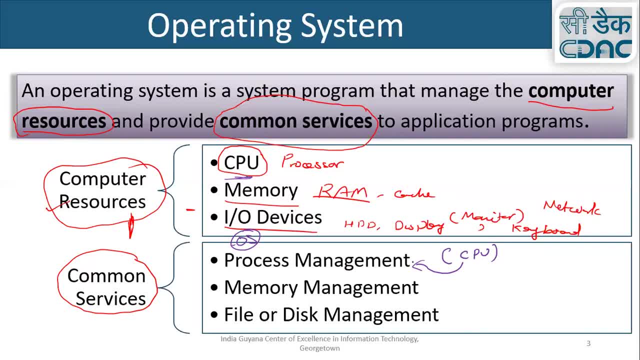 Manage the CPU. It's basically managing the CPU, your CPU, Okay. So that is the process management. memory management when it's managing your RAM? Okay. When it's managing your RAM, it's known as memory management. Okay. and What about this file or disk management when it's managing your hard disk? 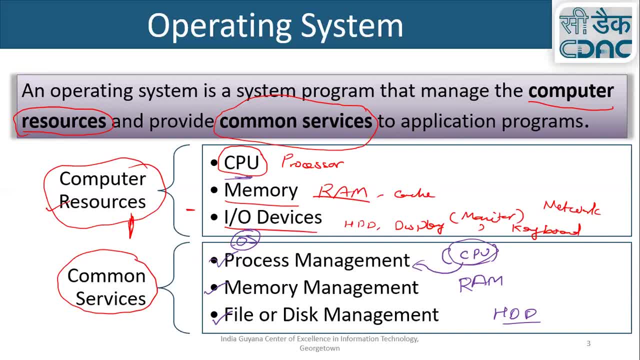 Managing the hard disk. Okay, So, while you're operating system, So managing the CPU is known as process management. Managing your RAM is known as memory management. Managing your hard disk is known as disk management. Okay, Today we discussed about this process management, this thing, okay. 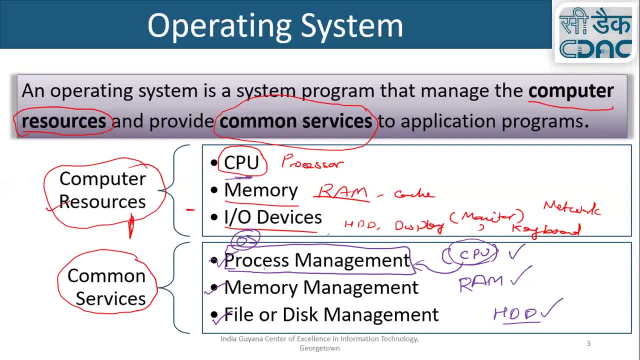 So what is the meaning of process management? basically, here we deals with your CPU. so, Inside the process management, What is the resources? This will set my resource to CPU, Okay. what are the services? Services related to process management is provided by the operating system. Okay. 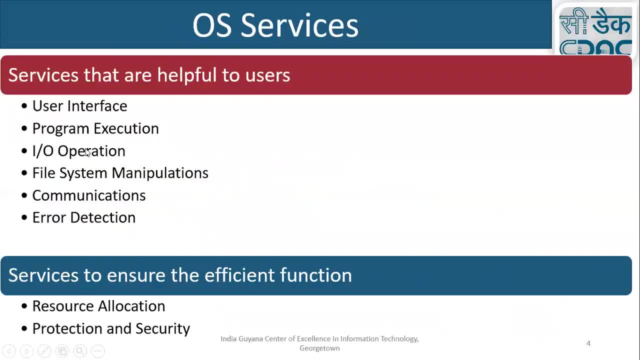 Good, Let me move the next slide. so, Before moving, what are the different services provided by your operating system? so your operating system provides you a Nice user interface, Yes or no? Yes, sir, window provide you a user interface. it's, It's provided. some It execute your program by just clicking on some icon. it you can execute a particular program because 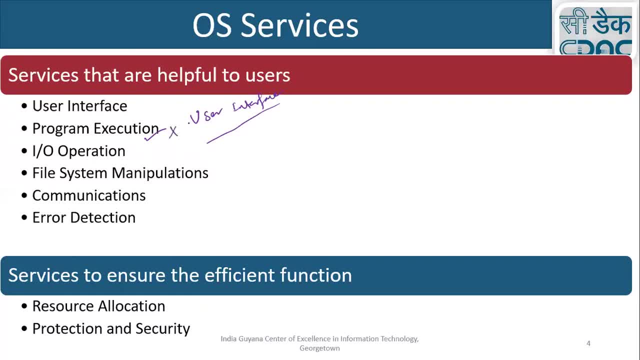 if it's not able to execute some program, then operating system is just useless thing. Okay, and then it you can perform some input output operations, like copy Kitchener's with diet. So I'm moving something from one location to another location location. so these are the io operations. similarly, the file system manipulation from one directory. 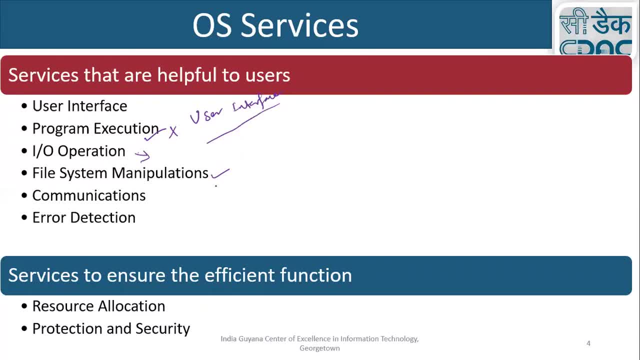 one folder to another folder. so we go deep in these things. and then my next presentation- uh, communication is related to your network things- and then if some error happens, it gracefully it's not just shut down your system, it just please show you the error message that something went wrong. 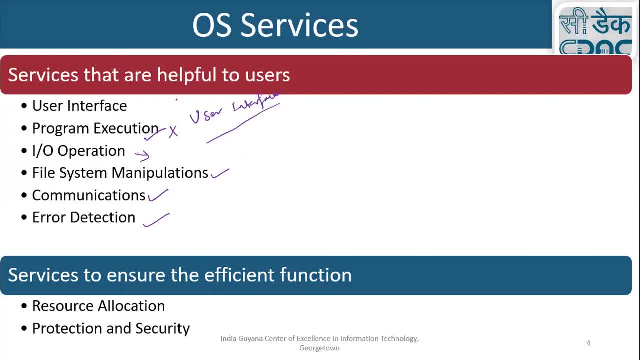 okay, so these are the different services as a user we get, okay, and then services to ins. so these are some helpful to the users as an end user and then to efficient function after computer system, remember, operating system. one name is also defined as a resource manager. okay, why operating system is also known as resource manager? because 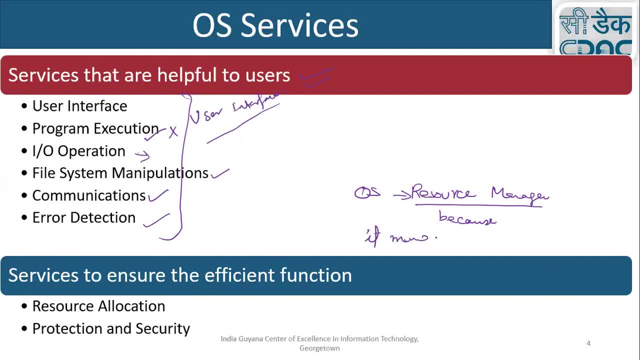 why it manages the resources. yes, okay, because it manages the resources. so so, these are the sub services. and then how? if you managing the resources, it's very important that you focus on the efficiency of those resources also. yes or no? yes, sir, if you are managing, if 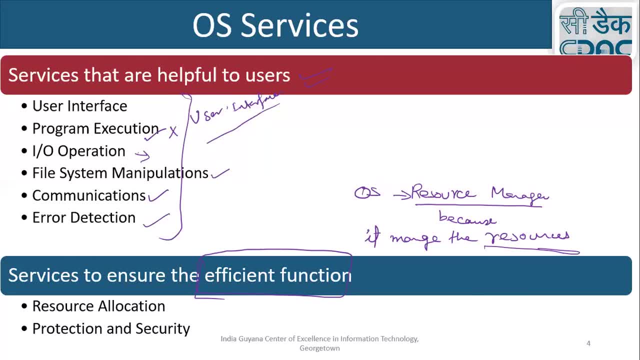 suppose you are a manager and you are working under your uh management. four or five persons working so you must make sure that they are efficiently works. so operating system manages a lot of devices. so it's the responsibility of the operating system to efficiently manage these resources. so how it's managing these things like resource allocation, 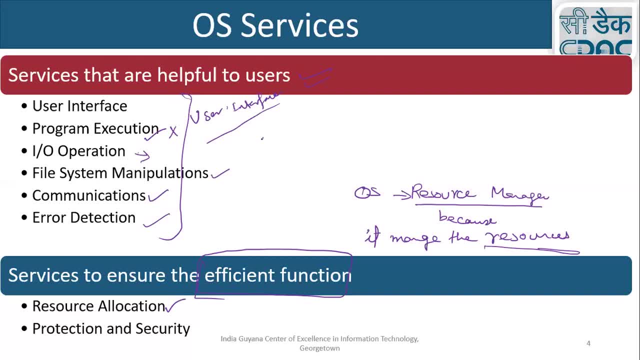 how much particular results? what are the resources? resources are your cpu, your memory, okay, and then your cpu memory, uh network network or some input output operation. so these are your different uh resources. so these resources allocated to the different programs. so this resource allocation should be efficient and this 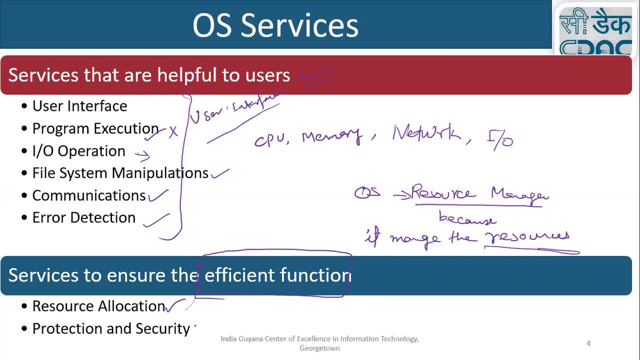 is the one role and next is the resource allocation. so this is the one role and next is the resource allocation. so this is the one role and next is the resource allocation. so this is the one role, and next role is protection and security. role is protection and security. 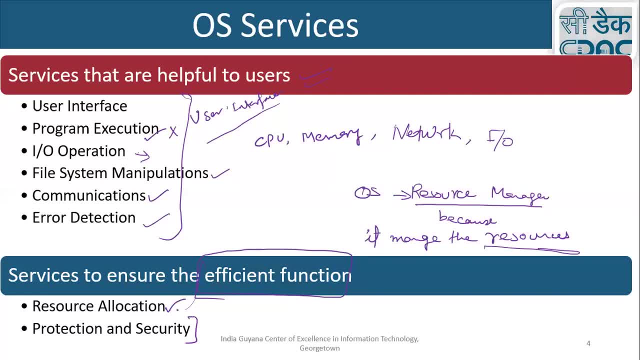 suppose you are using your system and it's automatically delete all your data. so that is not a good thing. uh, earlier in the window, you may not know, but earlier in window 98. if you heard about this, window 98 or not, yes, i know what. windows 19, yes, so window 98. 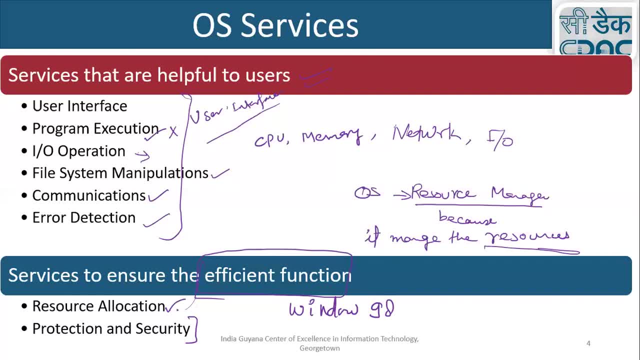 is in these systems. um, it happens a lot of the time that you just are using and you're all the data is gone. nobody know where is what happens. so now the systems are more gracefully showing the things what is happening. so protection and security is one of the uh. 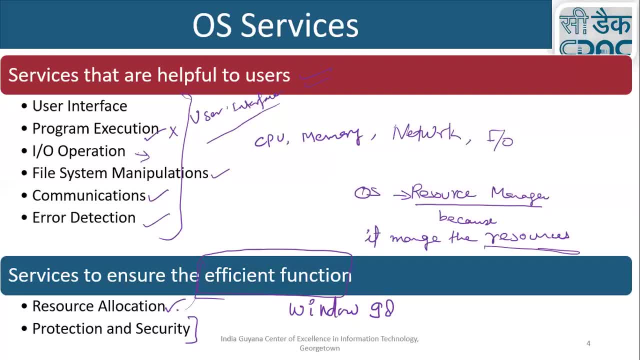 things that is provided by the operating system. so these are the different services that operating system provides. okay, some of these services is provided to the end user like user interface and just by clicking or moving files and directly from one location to the another location. so these are the some services that end user gets. 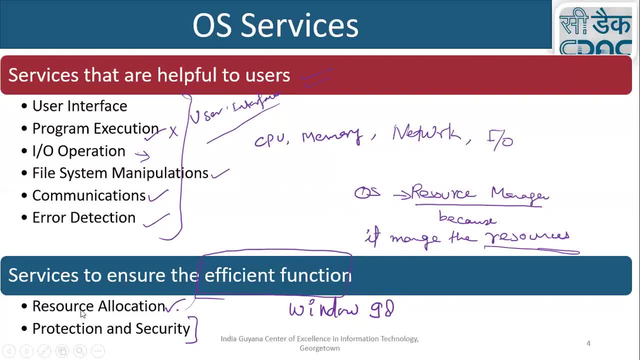 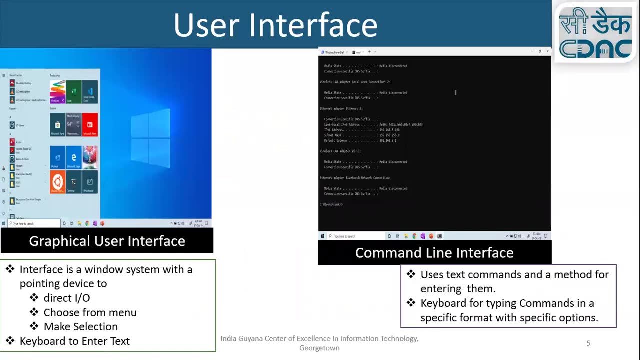 and then, under the hood, it manages efficiently, managing your all the resources and provide you the protections and security. okay, yes, sir. so let me move to the next slide. okay, so, uh, let me start discussing about the user interface. okay, so, this is known as graphical user interface or gui. 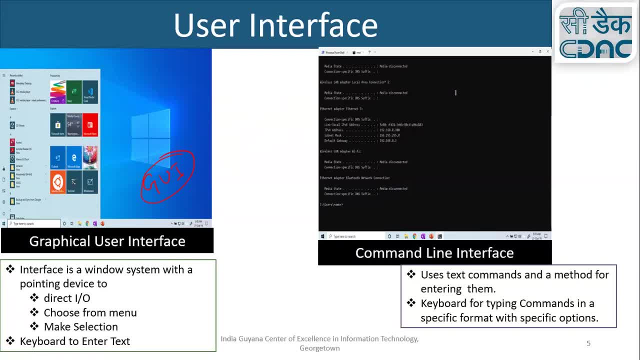 most of the time, uh, we just using the gui or graphical user interface. but uh, even the window is providing you a command line interface, or sometime known as cli. okay, so what is this? graphical user interface is a window system with a pointing device, so direct input output by just. 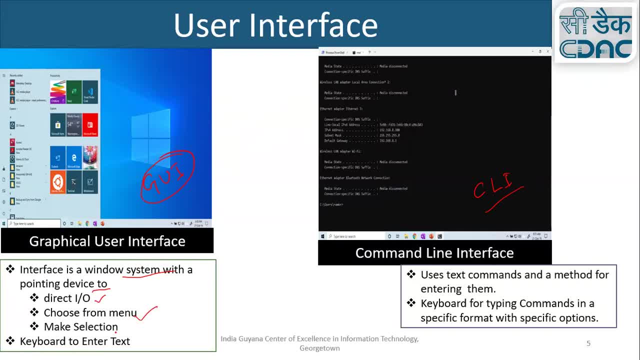 clicking your mouse, choose your device and then you can use this interface to choose from some menu. make selection keyboard to enter the text. you can use your keyboard to enter some text. okay, so these are the things your graphical user interface provides. in command line interface. you just have to write. 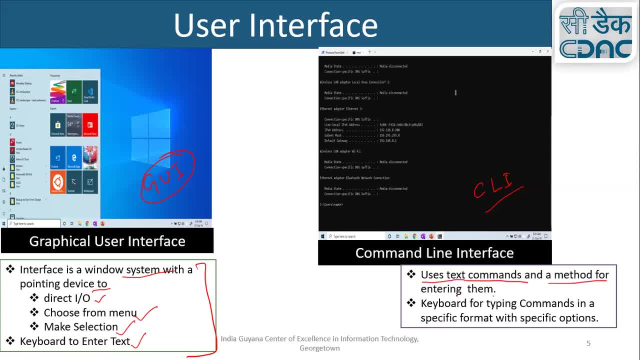 a command and a method for entering them. okay, keyboard for typing commands in a specific format with specific options. okay, in a nutshell, what these two things are doing in graphical user interface. you have to have icon for all the things like here: you have icon, you have icon, you have icon and you have to just click on these. 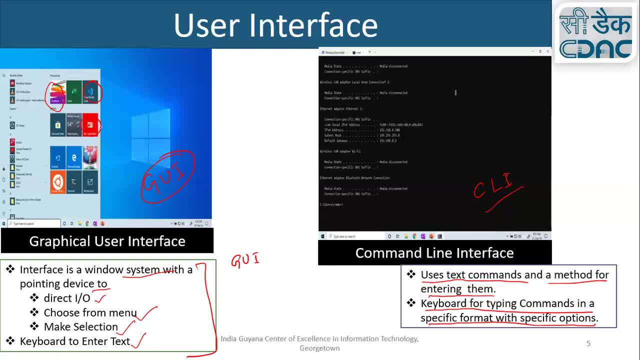 icons and that's it. once you click, you get your uh means particular program opens. then you can type something. what, whatever you try to do, you can do in command line interface. you have to remember the name of these gq table files, okay, so you must have to always remember these. 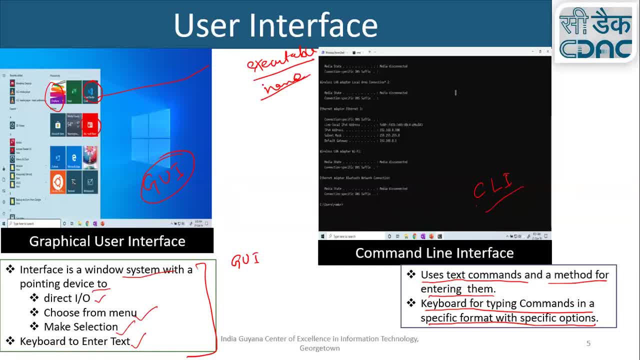 names. that's the one problem in command line interface. therefore, a lot of people try to avoid this command line interface because for everything, you must remember actually what command you can use. okay so, and remembering a command that is a text name is a difficult thing, instead of just clicking at some. 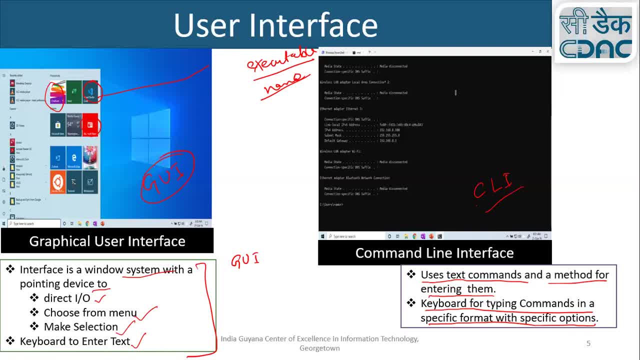 particular icon. so therefore the graphical user interface, uh, prevails. so a lot of users utilizing this graphical user interface and command line interface is just some poor developer or computer scientist, but they are using this command line okay, because a lot of people try to avoid this command line interface, because they have to remember these. 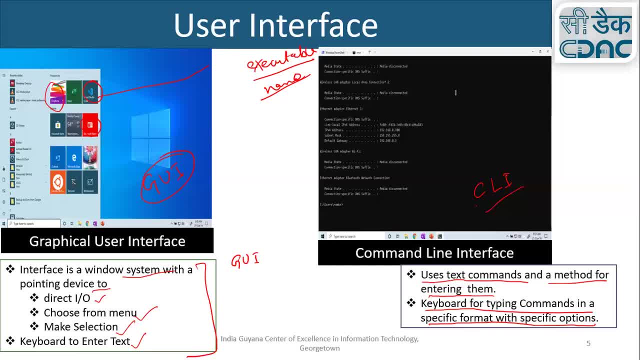 text command. okay, i'm just giving you examples. you have a program named ping in the study section i am discussing. so ping is try to find this. are these two things? your computer has? the internet up or not? internet up or down? okay, if you have a icon, suppose this is your icon for. 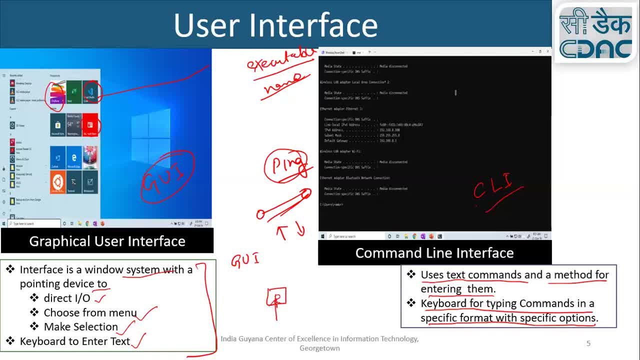 ping command. clicking on this particular icon is an easy thing for a new user. then, remembering this thing, open the terminal, a command prompt, and then writing this thing, yes or no? yes, so for beginners this thing is easy, but But if you can use this thing, because under the hood, when you click on something, actually these both things are the same. 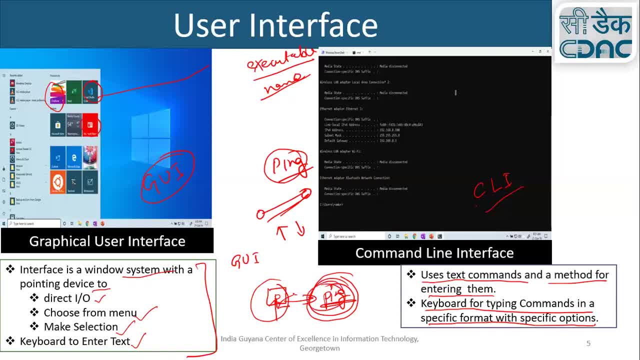 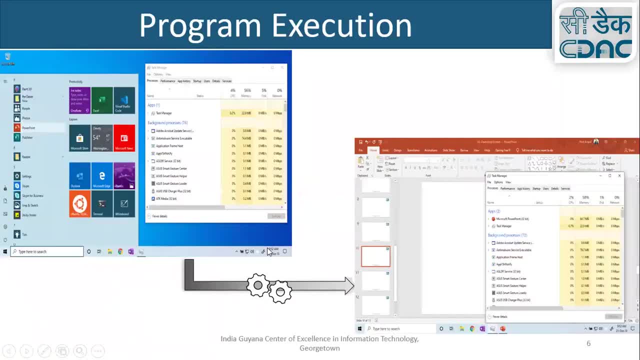 but Remembering this is a difficult thing. I will give you some, a lot of more example in other classes. Okay, Let me move to the next slide. okay, so I Am coming out. Let me complete this thing here. So what in this figure is depicted is this: try to figure out this part. 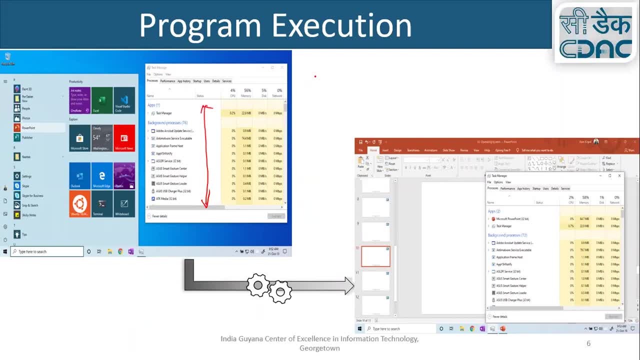 Yes, there is no powerpoint. Okay, It's related to program Here. I open my Start menu and click on this powerpoint icon. Okay, This thing I put at this place and my this is my task manager. Okay, so in my task manager there is no powerpoint. program is running currently and I open my start menu and 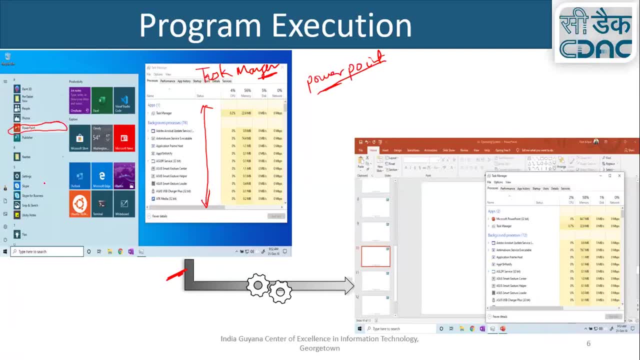 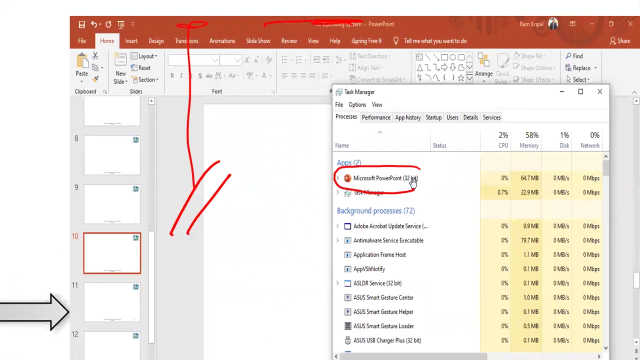 Just click on this powerpoint icon. What happens? this powerpoint Window open, Yes or no? This is a powerpoint window, and see here This part. Let me so is possible. See, yes, this You see. Microsoft PowerPoint 32-bit. It's utilizing 0% of the CPU because currently it's just. 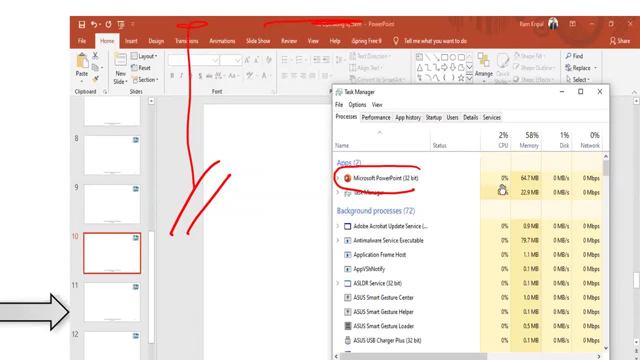 Open and I'm not doing anything here. So see this: CPU utilization: 0%. How much memory it requires: 64.7 MB. How much disk space it requires: 0 MB. network: No network: 0 MB here. Okay, so this particular process, so see. 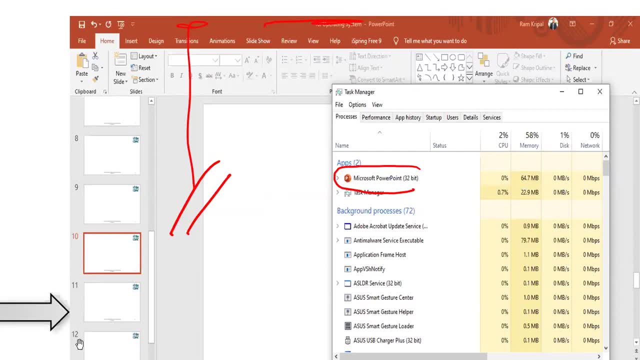 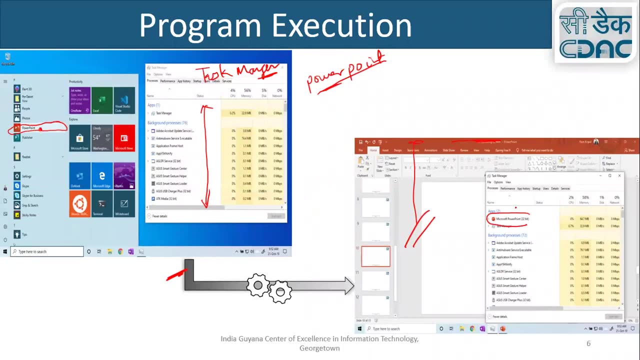 Let me zoom out. Okay, so when you click on something, some icon, what happens? These different resources are located like CPU, memory, Disk or network, okay, and these things are allocated by whom? by your operating system. So when you just click on any icon inside in your window or GUI, 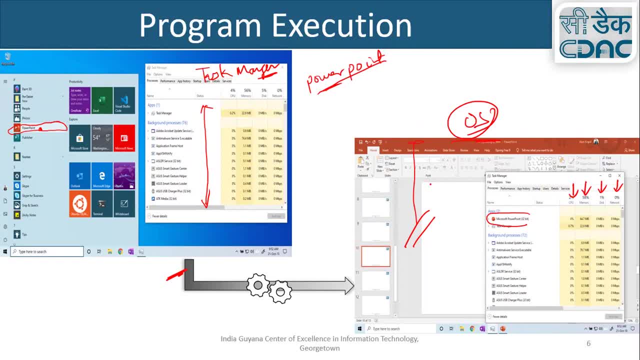 your operating system behind the scene, allocate the CPU memory network To that particular program. Okay, So please. and one more thing: rip I am just giving at this location here, here This thing is known as program. Okay, this is no nice program. PowerPoint program. Well, One note. program for word, program, any program. 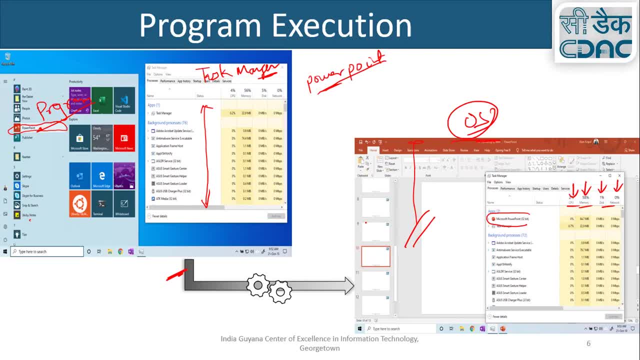 Once you just double click here, and when the program is moved at this task manager inside of that manager, It opens. when this window opens is no more each program. It's no nice process. Okay, Please remember this thing. when it is program. when it is, it is as: 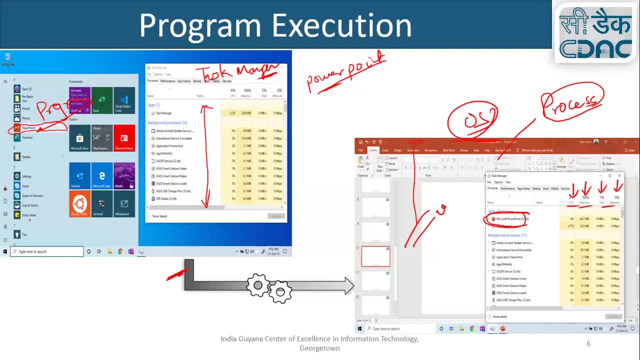 just stay inside your disk, it's not executing, then it is known as program. once it gets your cpu, it move to main memory. it's become a process. so program means uh. program means idle entity, okay, yes, sir. and process means this is active. once it is active, this is your process. okay, so let me move to the next slide. 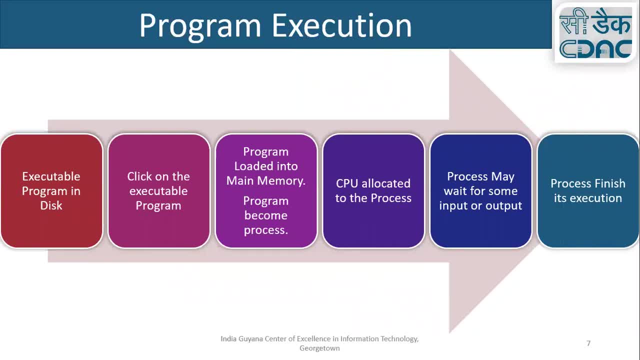 okay, so how this program executed. so at the very first step. uh, your pro, okay, when you click at this. okay, suppose you have the powerpoint example. i'm taking this. this is your powerpoint icon, where it is. if you just right click and go to the location, it is. 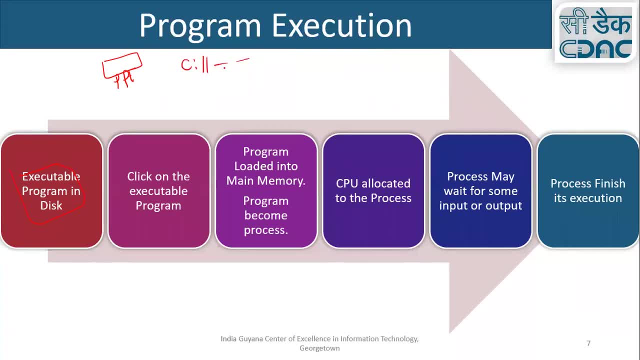 stay inside your c drive, yes or no? see that. and sublocation. so normally your executable programs is inside your exchange at this your hard disk, okay, and then you double click on this particular icon, you click on the executable program, then this program from your hard disk move to your. 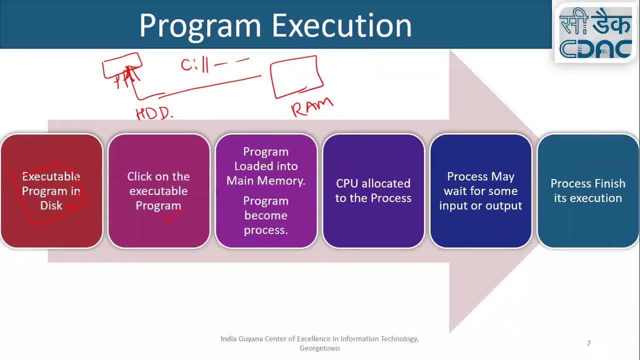 右 side of your, your main memory, you see it's loaded. uh, now, when this program is inside your main memory, it is named after the one of thehos, which is the magical ram or main memory. okay, yes, sir. so program loaded into the main memory, and once it's loaded inside the main memory, 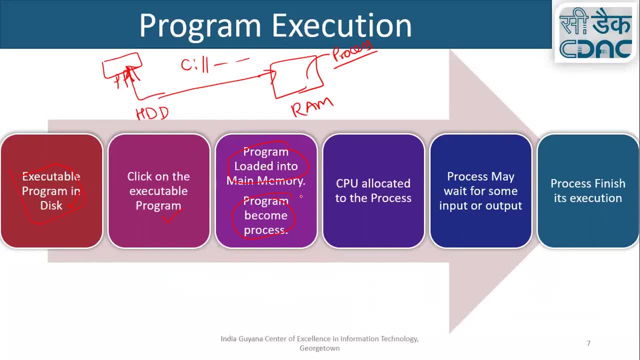 now this is known protest: okay, the CPU allocated to the that process. okay, because without CPU this program can't execute. so CPU allocated to that. so see a location is a resource allocation, yes or no? CPU is the resource, hardware resource is allocated to a particular program. so here you want process management. this is a process. 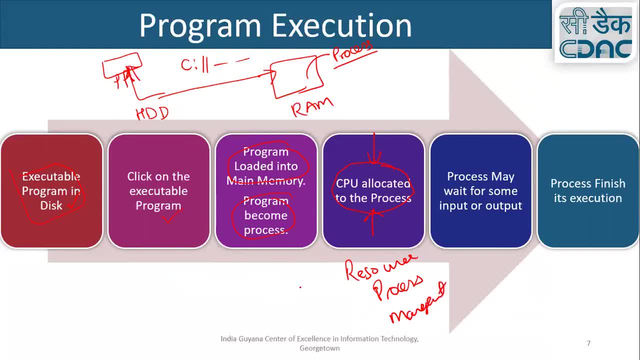 management, yes or no? yes, yes, program loaded into main memory. main memory allocated to memory located to your program, program. okay, main memory allocated to your program because program move to the main memory. so main memory allocated to the program. main memory is my resource and operating query allocating it, updating system allocating it. so our pitting system. 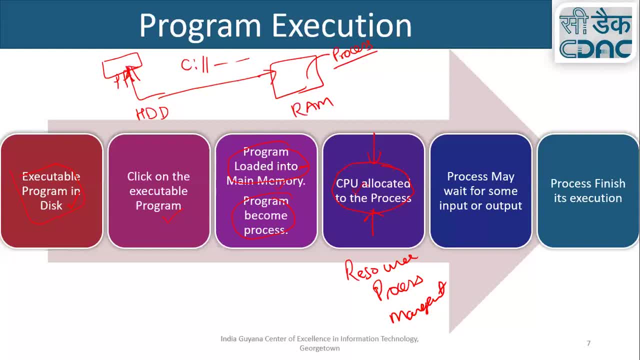 management is the ability of the system to control the implementation of the. manage this main memory operating system, manage this cpu. once the cpu allocated to the process, process execute, it may bait for. something like: if you open your powerpoint presentation, it's baiting for you write something. or if you get a new slide, do something. so process may bait for. 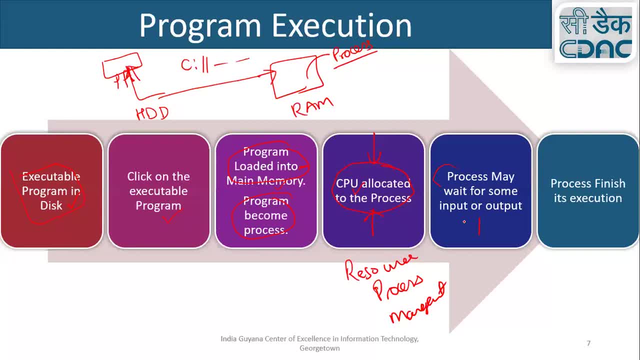 some input or output and once it finish process, finish its execution and it executes. so this is normal way of executing a program. you click on a particular icon that is inside your disk. hard disk programs move from your hard disk to main memory. it becomes a process process. get a cpu. 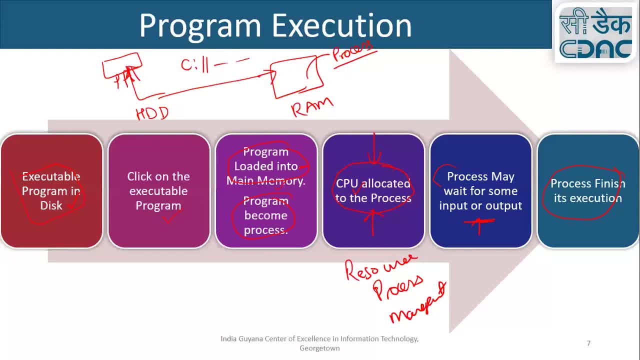 it may execute something and then it bait for some input or output from the user and, once it's completed all the things, it finished its execution and get out and release all these resources. this is main memory. this CPU is just written back to our particular getting the things, sir, in it. 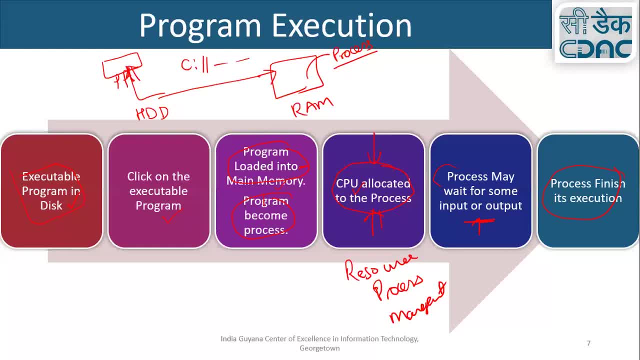 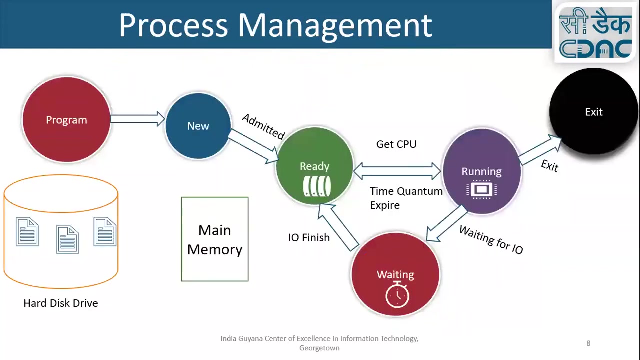 out. it's straightforward, because from the executable program it goes straight to a click on young, the program, it's loaded into the main memory and the main memory it becomes a process and then continues on to the CPU and allocates, and you know it goes on from here. good, let me move to the next slide. so here I 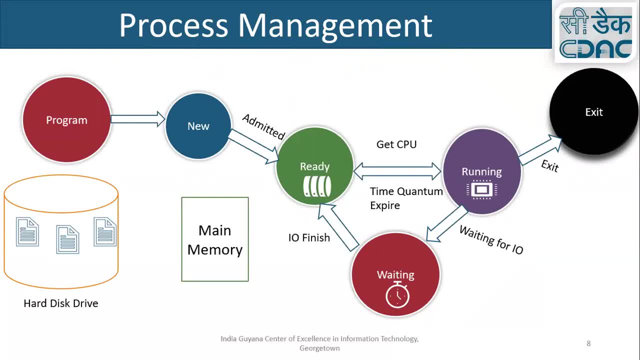 am just giving you the complete thing, complete picture. so this is your program inside your disk. okay, this is the step number one. okay, it's a program. yeah, you just click it here. okay, it goes to the main memory. okay, here's the main story. now it is no, right so? 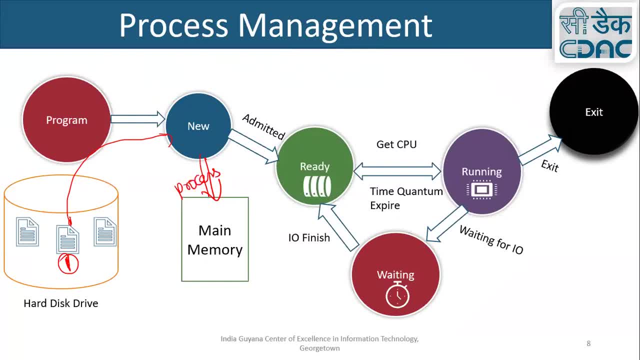 okay. yes, sir, now it's this in new shape: a be solid state. okay, and then okay. so it's not the only one program. your computer you can, you may open the multiple programs, it's not only one. maybe you have a program number one, program number two, program number three, you have a lot. 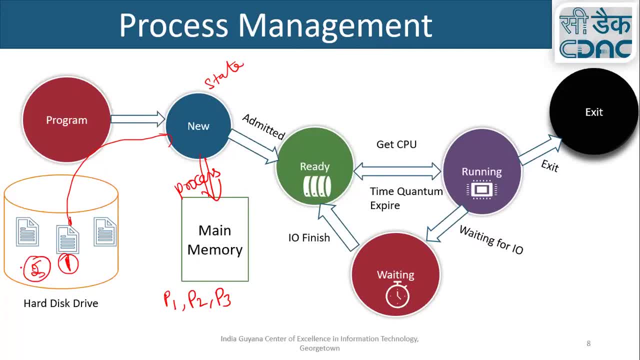 of program on hard disk and maybe you just click on the I program so these programs moves to main memory. so main memory have a lot of processes, because once the program moves to the main memory it's known as process. so these processes are baiting for your CPU because 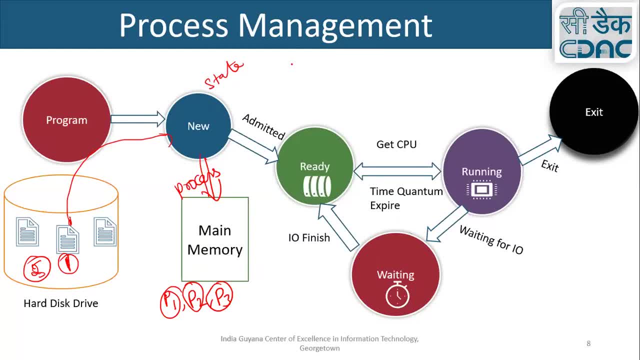 if okay, suppose you open the, your chrome, then your powerpoint and then maybe your browser, not browser, some media player. okay, so you just open two or three programs and these are the programs. without CPU they can't run. the CPU is exist at this place, so these are just in baiting queue. these are 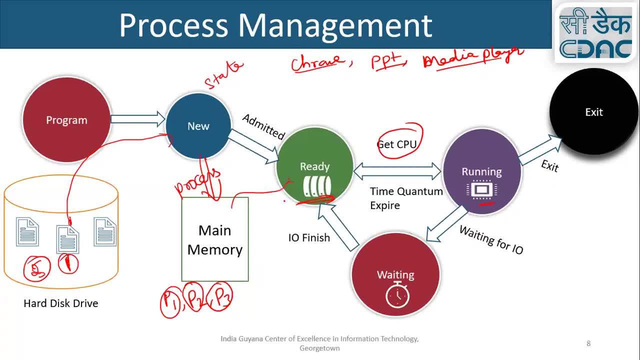 aligned in a queue. okay, so these are the processes. are just baiting, okay. and then then your operating system, take a particular process and give it a CPU. so while they are baiting for the CPU, they should know that they are in ready state, okay, they are ready to execute, but they don't have the CPU once they get the CPU. 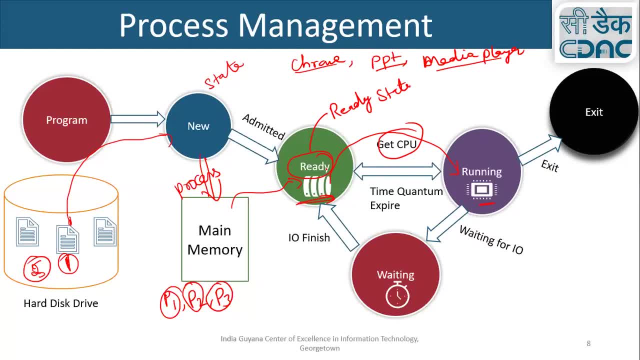 they move from the ready state to. this will move from the ready state to running state. we can now they get: yes, okay, if everything is normal, they complete their execution and then just take it. so what is the normal vision are you? you just click on a particular program. program becomes a process moving the main memory. 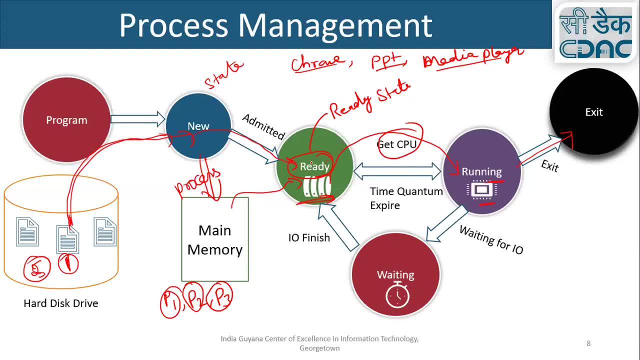 it's bad for your cpu, okay, it gets the cpu go in the running state and it finishes execution and exit. so this is a normal scenario one day. what are the other scenario possible? other scenario maybe: okay, if in the ready sir, yes, um, what is the time quantum expire? that was like the one thing. 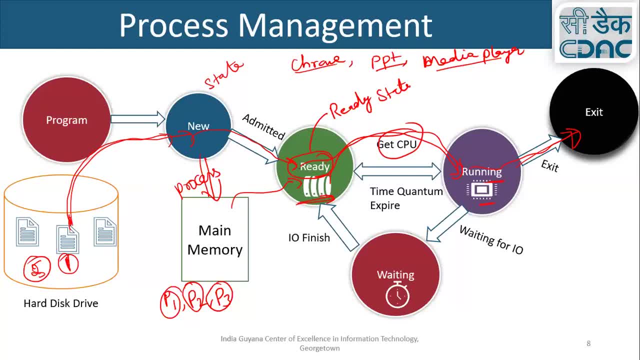 i'm, i'm coming, i'm coming on that thing, okay, so i'm just, uh, i'm just describing this particular pathway, this pathway, okay, get the cpu now. uh suppose, uh, this process, You start from here, go to the new state it's getting for your in the ready shape for the cpu, it gets. 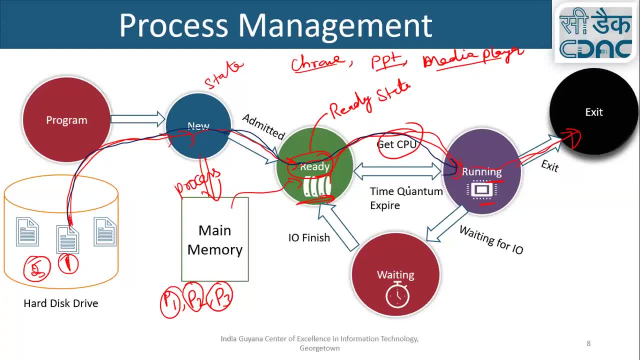 the cpu. okay, like you open a powerpoint and then you're just not doing anything on the powerpoint, just open it and leave that. so how long the if your operating system allocated the cpu to this, your powerpoint thing, your powerpoint presentation, and you are not doing anything. so no, okay at one. 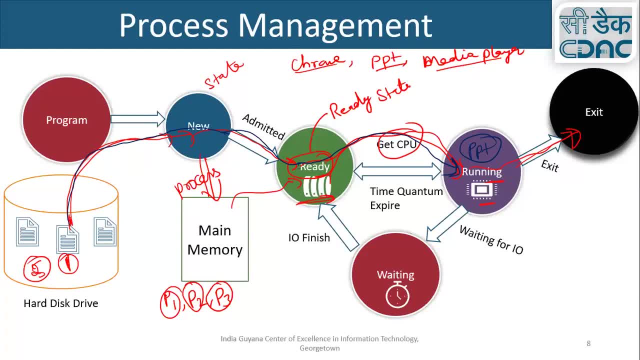 time only one process can run. if you have only one, four. if you have four, four, you can execute four process. okay, so if you don't have, suppose you have four calls and you have opened up eight processes and your powerpoint is number seven process, it get a cpu but you are not doing. 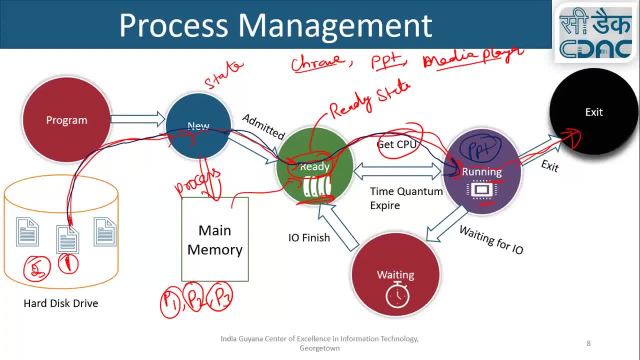 anything. so your cpu's time is just wasted, yes or no, because it's useless. you allocated a cpu to a particular process and that process is doing nothing, it's just waiting for user input. so at that point what happens? your operating system remove, move that particular process in the 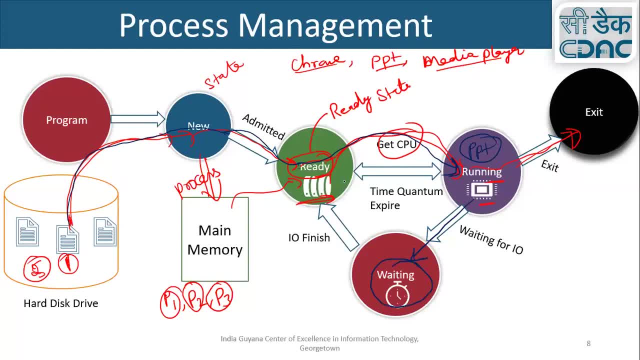 state okay and it allocate the cpu to some other process and once its input output is completed, whatever thing it's getting which, once it's completed, it move to again in the ready state okay and you again get the cpu. so it may be that they move in this particular cycle here this day in this cycle and once it's finished things it get. 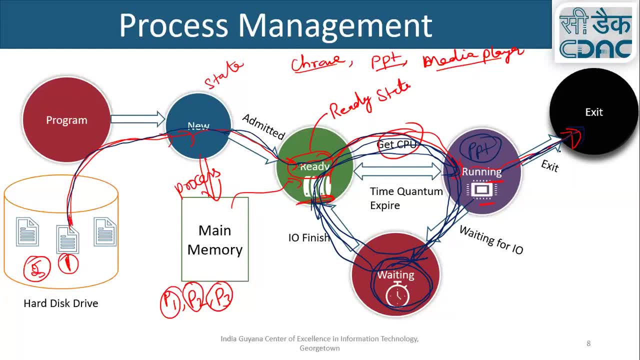 out. so this is the second possibility. okay, good, so first possibilities. program. you click move to in the new ready main memory from main memory. it go in the queue. i bet it's waiting for the cpu. it get the cpu, hello, uh, and it executed its instruction and eject. another one is that it moves from the disk to main. 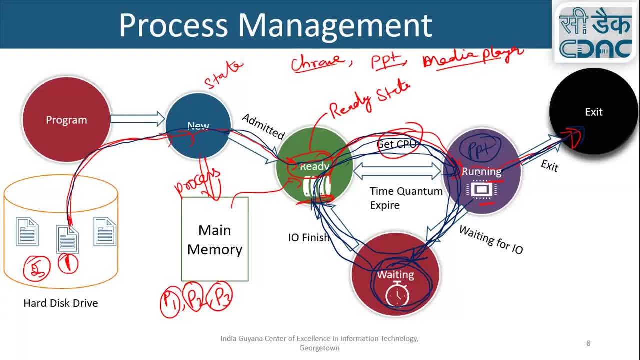 memory. it's ready for the cpu. it get the cpu, but it's taking too long for some user input or output. so your operating system move this particular process in the betting state where it completes its input or output thing and then it moves from the disk to main memory. it's getting the cpu, but it's. 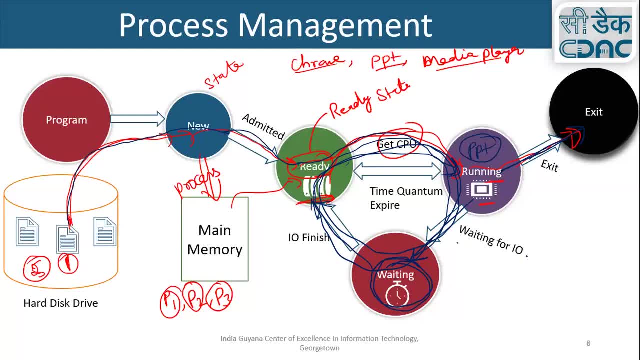 then it once it's complete. so they see, here it's betting for some input output and here it finished its input output. so once it's finished this input output, uh instructs operations, it just move in the ready state and from the ready state it again go in the running state. it's completed its operations. 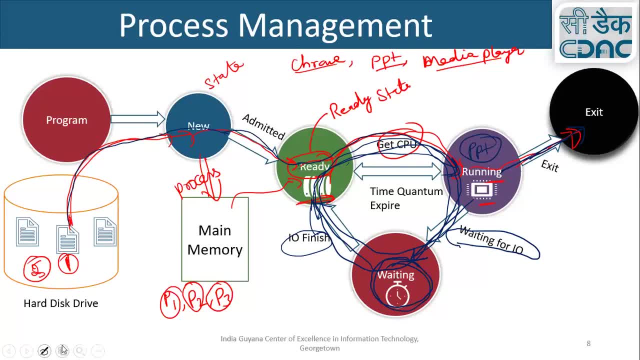 and eject. so this is the two possible way. now let me uh take some other colors. i think so that. so this is the two possible way. now let me uh take some other colors. i think so that is a pistol. so now, what is this time point, something, okay. so suppose you are executing a program. a particular program suppose takes 10 seconds- although it's a tool means it's a huge time. but suppose p1 takes 10 seconds and you have p2, p3, up to 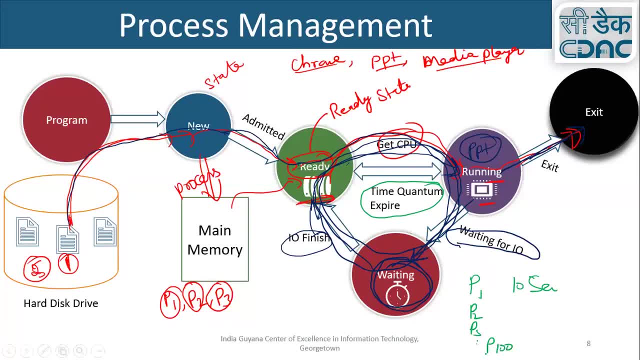 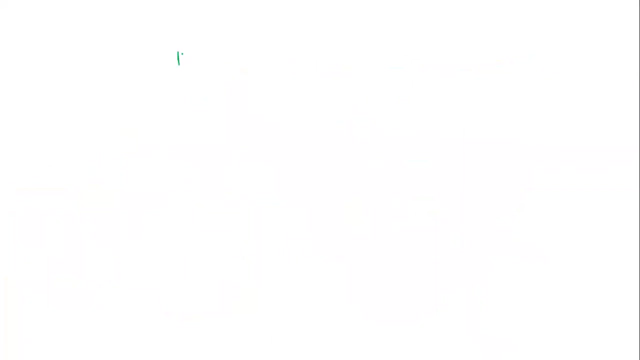 t100. These are the programs. takes one second. Okay, You're getting my point or not? Somewhat you could continue. it did. okay, Let me open up Why district here. Suppose you have a one program, p1, that takes 10 seconds, Okay, and you have a 10 more program. 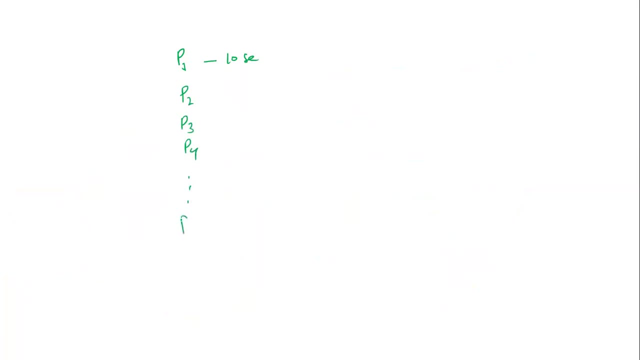 Suppose You can. these are the programs. take one second each. if Somehow other, this particular process p1, Get the CPU. Okay, if they locate CPU is allocated to this particular program p1 and if you start physically, then these are the programs. are better, Waiting for how long? p2 bit for 10 second, then this bit for 11 second, this bit for 12 second. 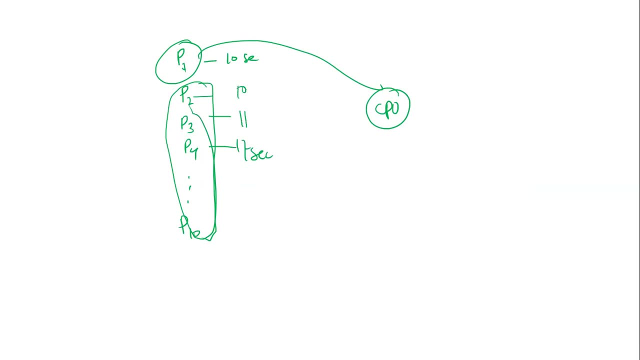 I'm so much yes or no. so, Generally, what happens if a particular process that has long execution time? If it has a long execution time, Then these small process are bleeding part very long time. Yes or no, like if you go in the bank. Yes, and 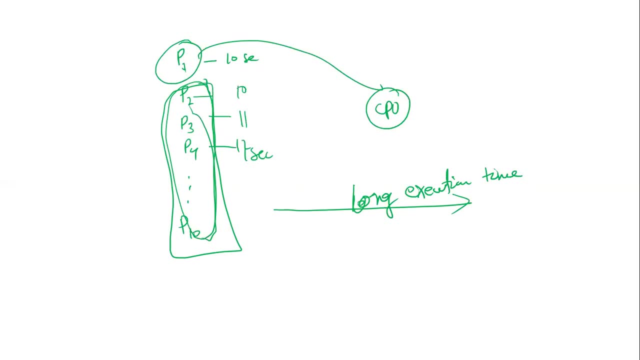 person Which is suppose you go as a bank counter. Okay, so here This is a bank counter, If this is an employee serving all the people and you have one person here in the queue, here, one person, here, one person. these are all the different persons inside in a queue. 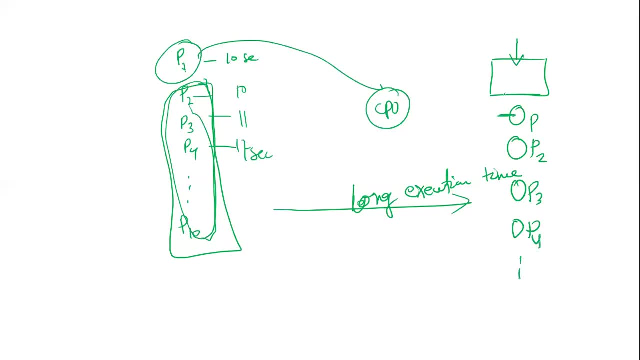 Okay, And suppose this particular person serving this particular person takes one hour? Okay, What these people say? These people say: I just need one second, please do my work, and then you, just in between, you serve this particular person because this particular person is taking too long. 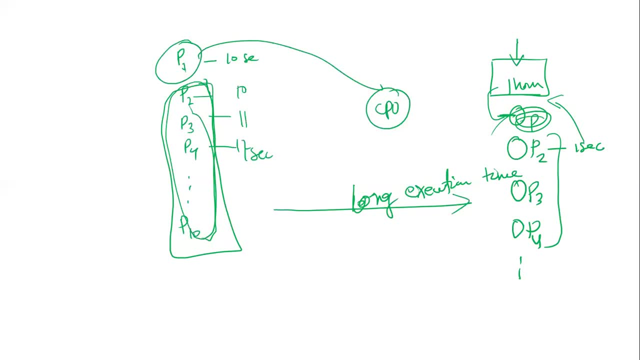 Yes or no? Yes, You are getting my point. Suppose the person who is in front of you. he is taking one hour and you have just one minute work, So you just request that please give me one minute. complete my job and this person requires. 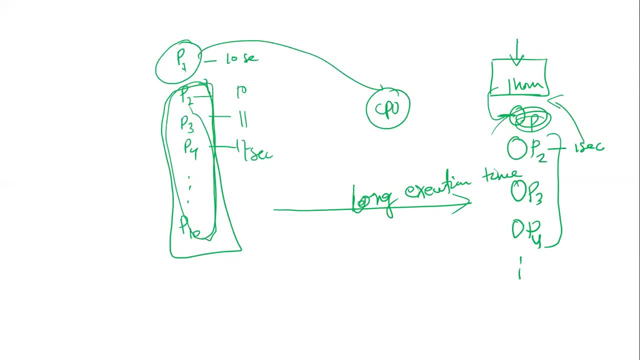 one hour. So after me, just give me yes or no. Okay, Yes, sir, technically, because you your thing would already take long and your thing taking long, so it wouldn't really make sense to you to wait that long when it's just a. 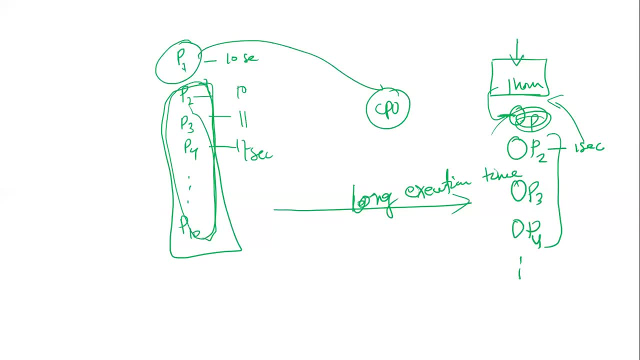 one minute, something you got to do. Yes, So, not. so. this is a particular algorithm in, yeah, in operating system that is known as round driving. Okay, What it's doing it's something like this: It allocate a particular time, suppose maybe two second, or maybe when it's it's a. 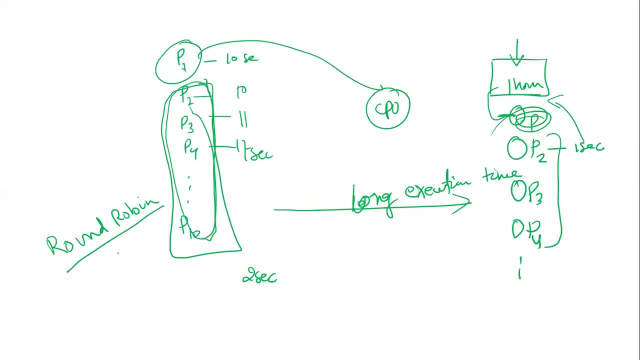 very small amount, not two second, very small. but I'm just taking example of two second. Suppose it so which is like this: it allocate two second to each process, and if that process finished in two second, good, So in one go it allocate two second to this process. so it just it require eight more. 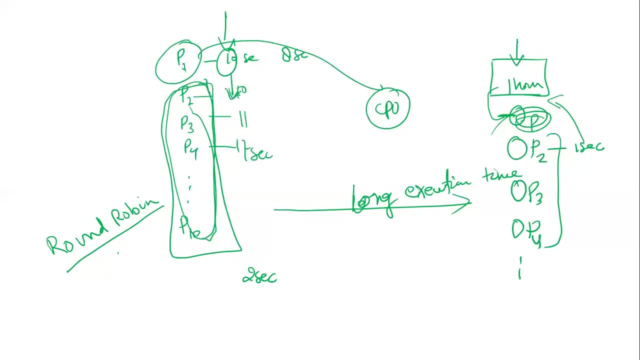 second, but it just move to the next process. Okay, It need one second it and here these two second. so after one second this process get out Okay And it move to the next process. So it maximum, maximum amount it give to a particular process is two second. 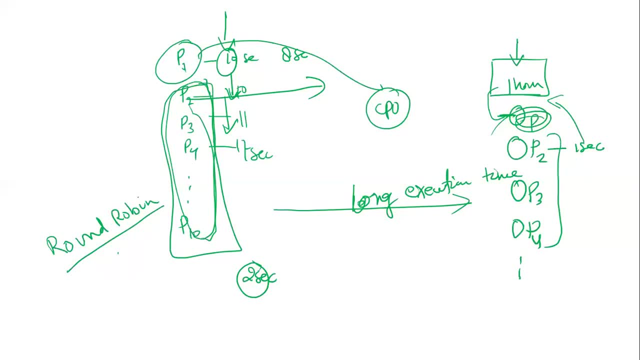 And if that particular process complete it's work in two second good, Otherwise just wait for next round. So that is the meaning of this round driving. It goes in round each time, just giving each process how much. 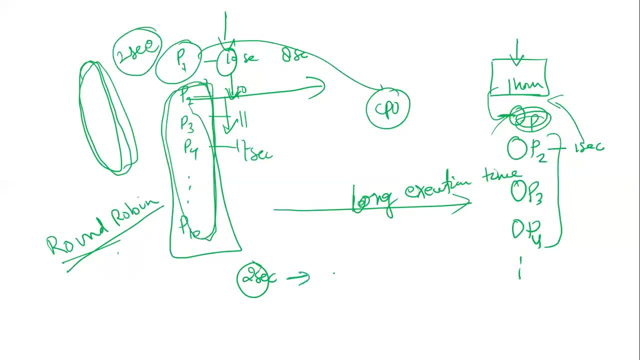 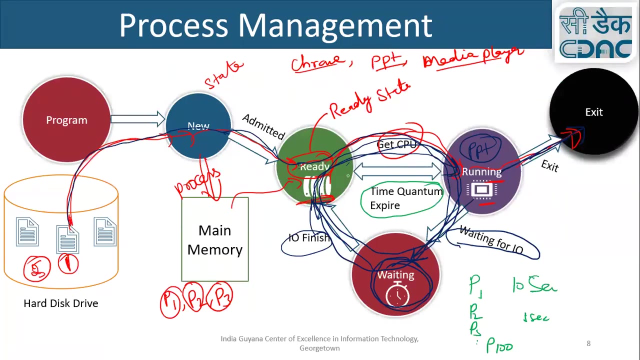 Two seconds, So this particular time, this second is known as time quantum. Okay, This is known as time quantum. You get the thing. So now see, now see this thing. So if the round driving algorithm implemented, if this round driving algorithm implemented, 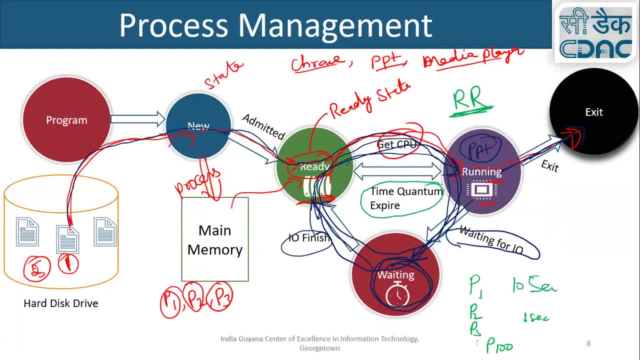 what happens? This process allocated to CPU and in running state. But if the time quantum expire, whatever the time quantum, maybe two second, two nanosecond or two millisecond- once this time quantum expire, this process will move from running. 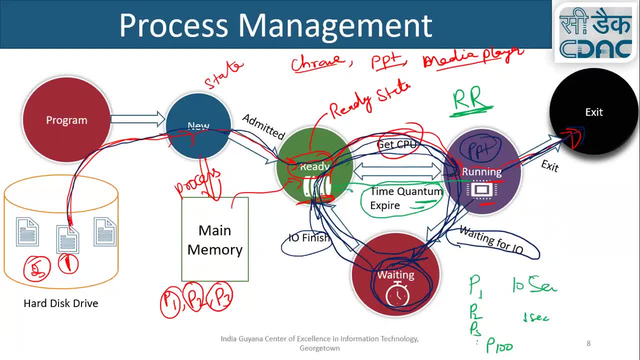 state to ready state And once it finish with all the process in the ready state, it again serve this particular process. Okay, So time, if the time quantum expire, the process will move from running state to the ready state. So that is the meaning of this: time quantum expire. 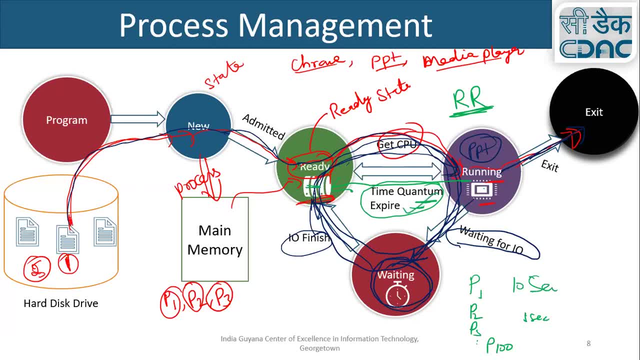 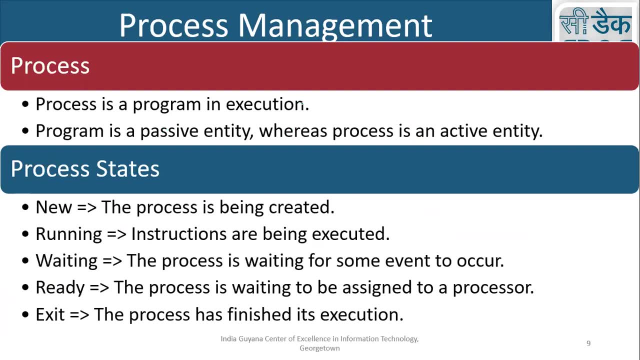 Okay, Good, Okay, Let me move to next slide. So what is the process? Process is a program in execution. It's already clear. Program is the passive entity, Whereas process is an active entity, It's just executing. Program is inside. 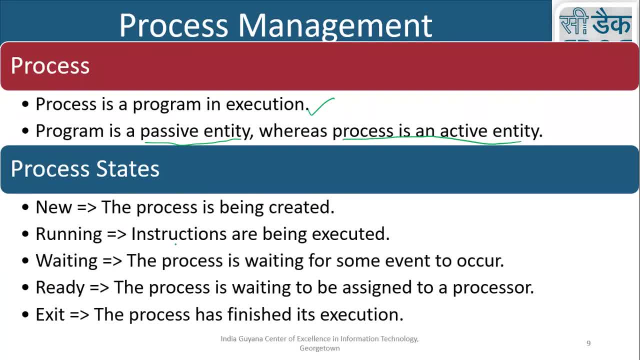 It stays on the disk. Okay, What are these different states? New, The process is just being created. Instructions are being executed in running state. Baiting means the process is baiting for some event to occur. These are the things. if you move in the previous slide, see everything is written here. 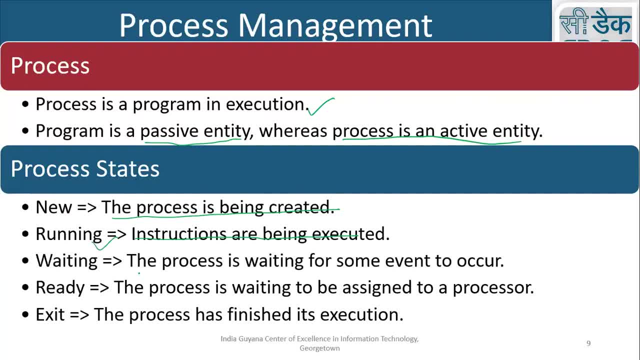 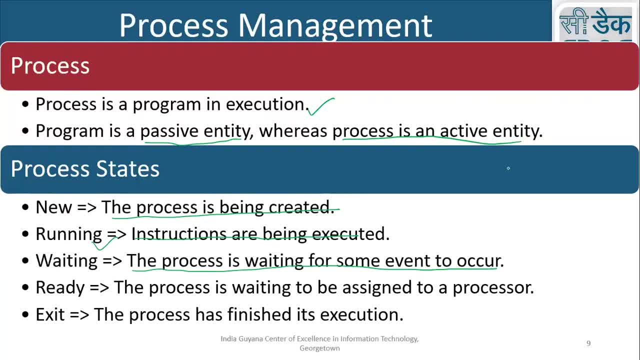 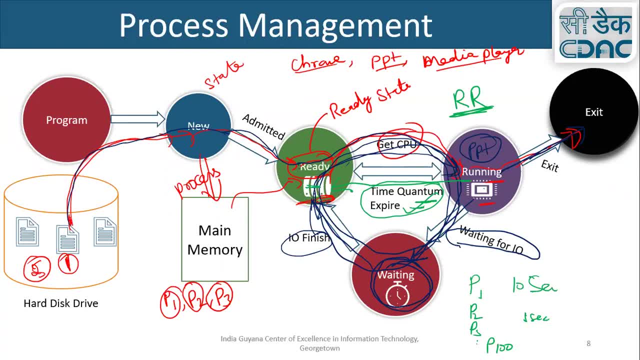 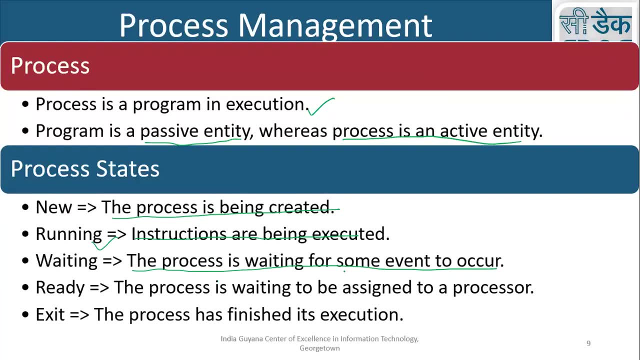